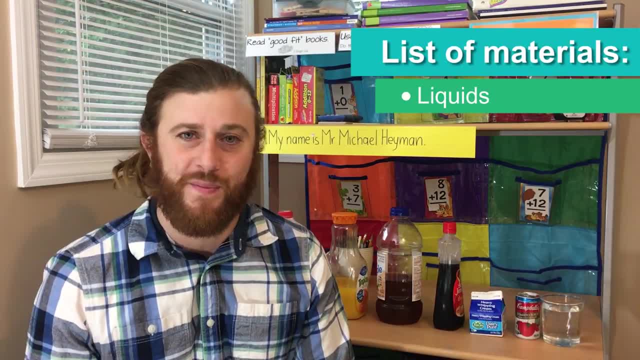 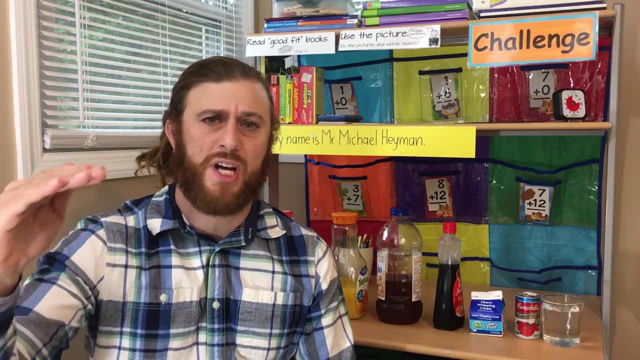 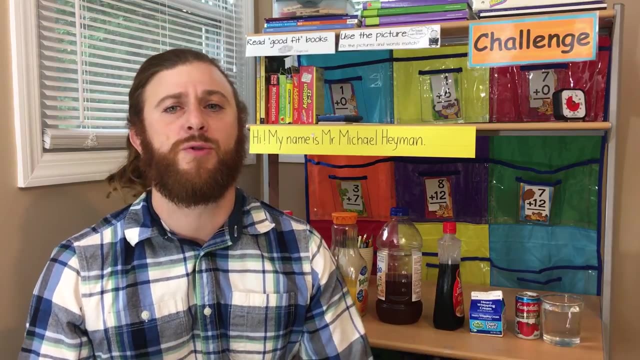 such as different liquids, an ice cube tray and a timer. While we conduct this experiment, we're going to follow the steps of the scientific method, as you should with your student or child at home or in the classroom. This experiment is so fun that it's an awesome teaching opportunity. 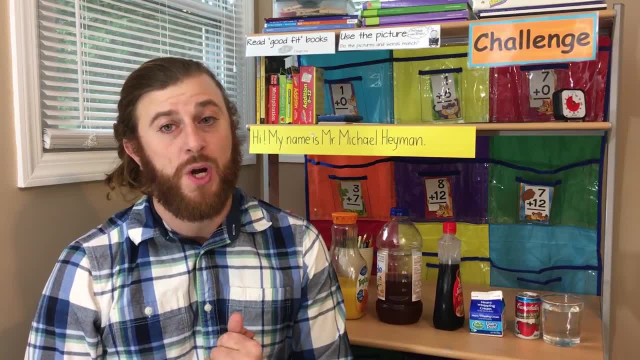 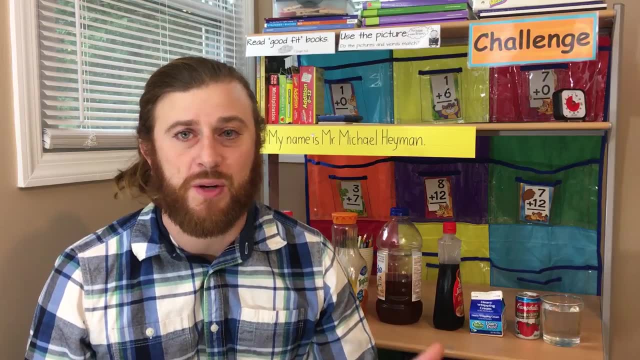 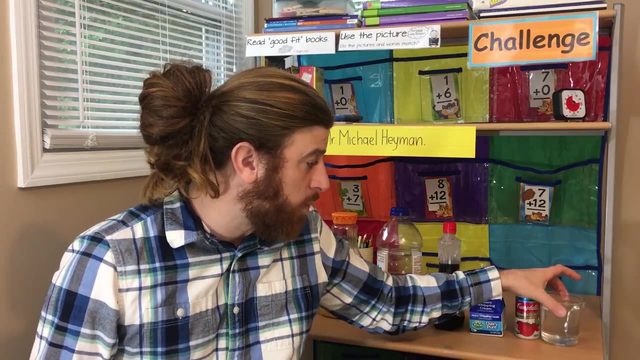 if you use the correct vocabulary and the correct steps when using the scientific method. Let's get started. The first thing we'll need to do is freeze some liquids. Now, which liquid should we freeze? You should always do something familiar, such as a glass of water. 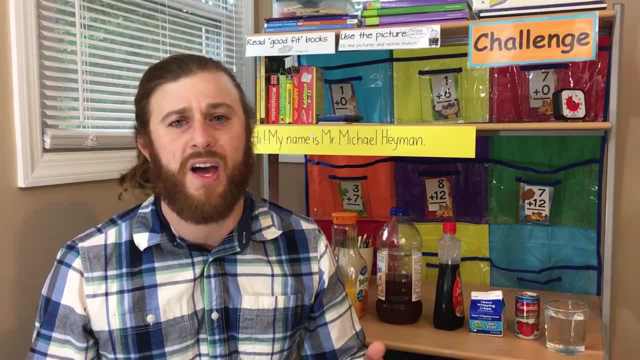 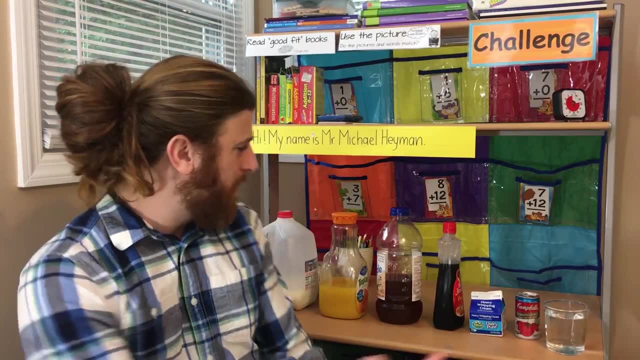 which will turn into ice cubes, so that you have something to rely on, some kind of background knowledge that you can pull. You'll always know that the water will freeze into ice cubes. What about some of the other liquids? Well, I chose some readily available liquids that I had in my refrigerator. 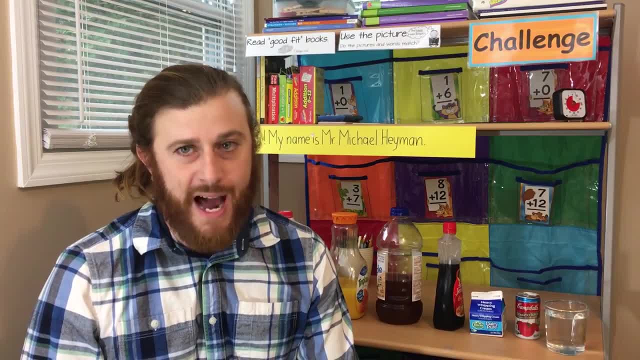 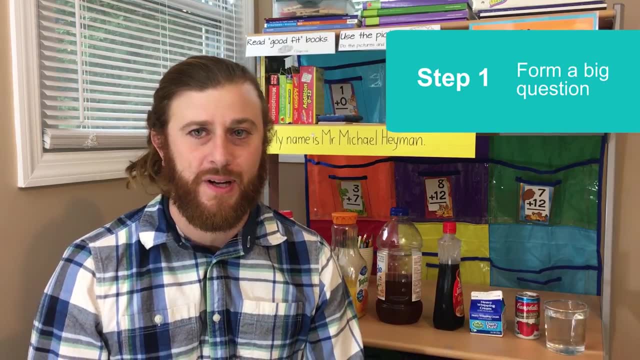 the same that you can do at home or in school. Now, after you've frozen these liquids, or even before, you should make a guess as to what's going to happen For your older students. you can ask them: do you think all the liquids will freeze, and why? 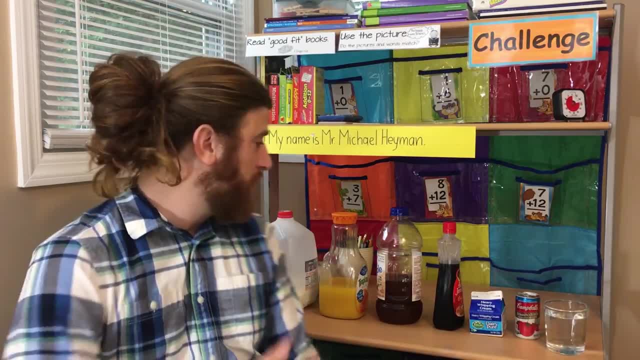 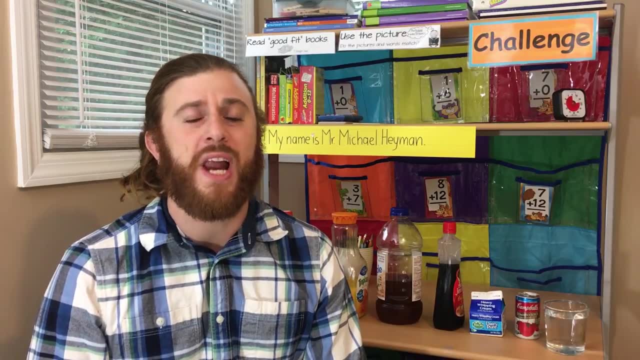 For your younger students, you should choose liquids that will definitely freeze, such as milk, orange juice and water. Once these liquids have frozen and again or before, you should ask them to make a guess. Third-grade students ask them to form a hypothesis. 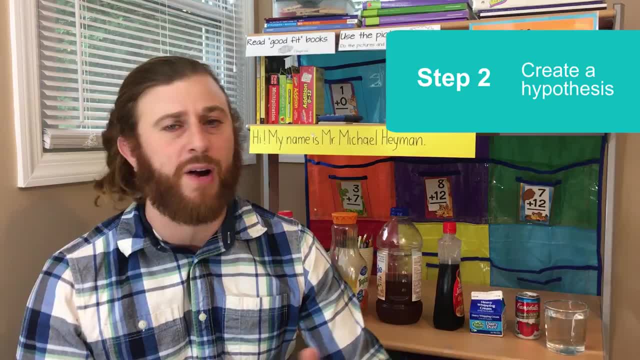 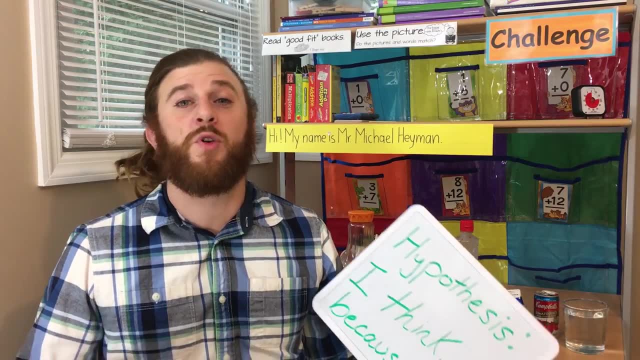 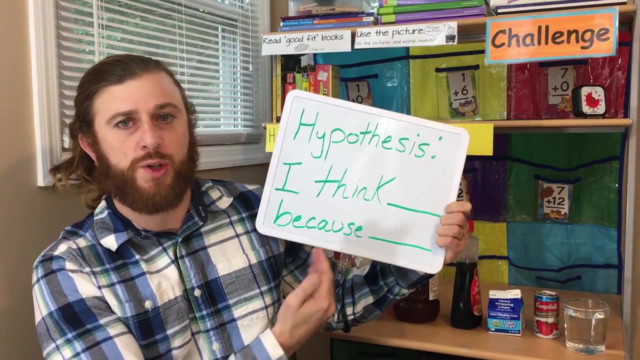 The older students should base their hypothesis on some sort of background knowledge and the younger students should try to pull on some knowledge that they have from the world around them To form a good hypothesis. all students can use the sentence starter. I think blank because blank. 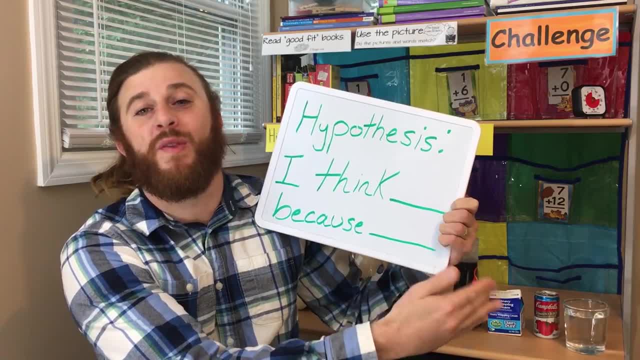 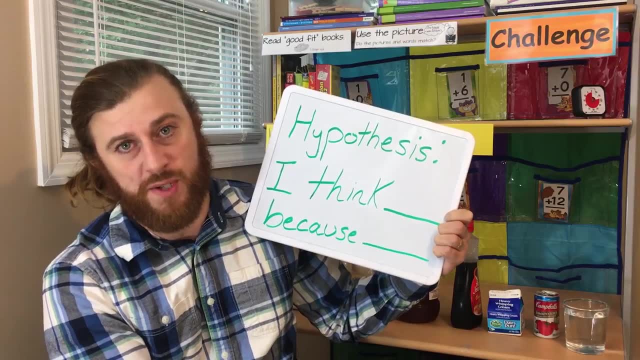 For example, I think the milk will melt the fastest because I've seen ice cream melt in the summertime and I know ice cream is made of milk. That's a good example of a hypothesis for about a third grader. They're using some of their background knowledge. 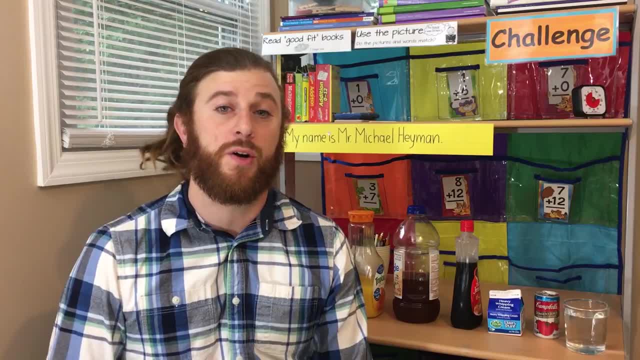 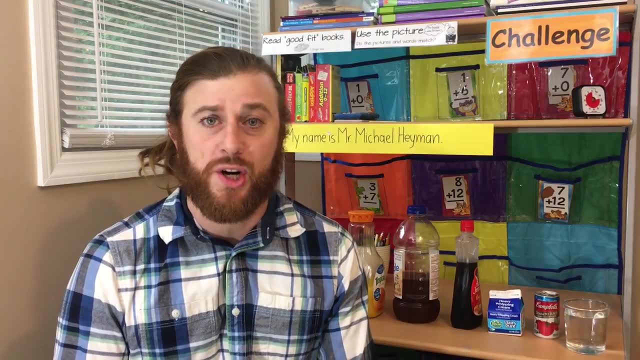 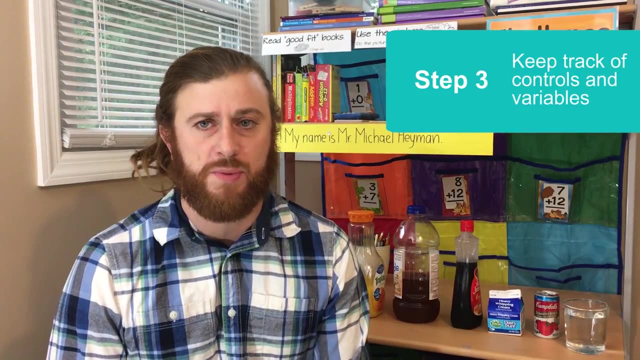 to help them form this hypothesis. Don't expect a kindergartener to come up with something this complex. Next, you'll want to discuss some other things about conducting a good experiment with your students, such as controls and variables, One control that we'll be using during this experiment. 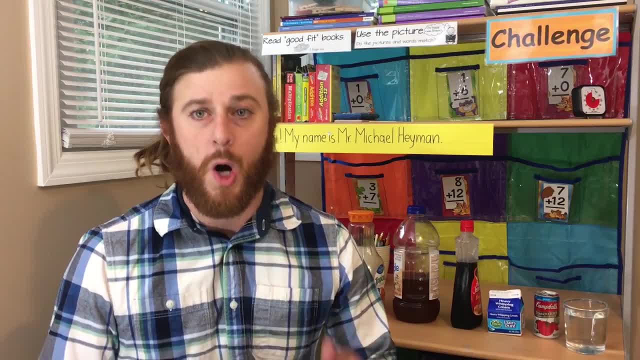 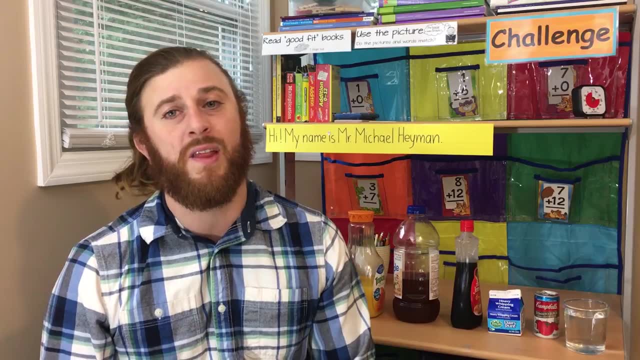 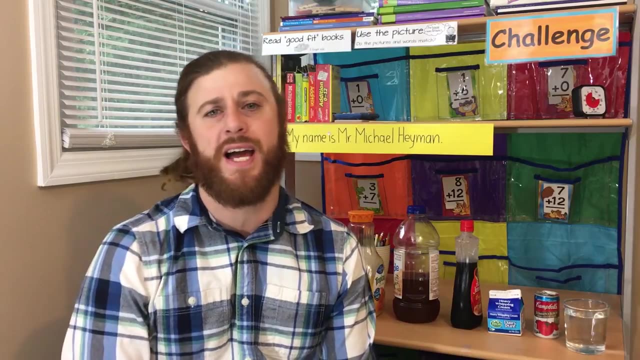 is the temperature in the room that will be melting the cubes. All the cubes will have the same temperature around them while they melt. We will be controlling this rather than letting it be random. Another thing that we are controlling is that we have the ice cubes that are exactly the same size. 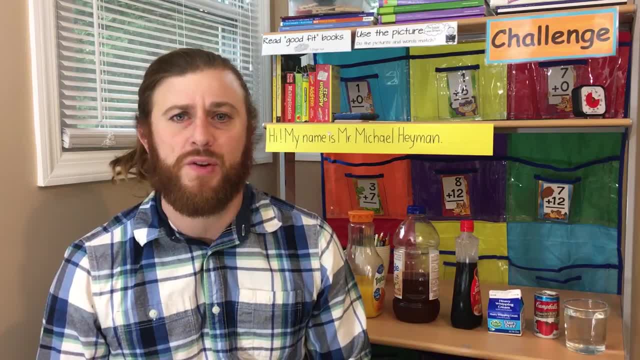 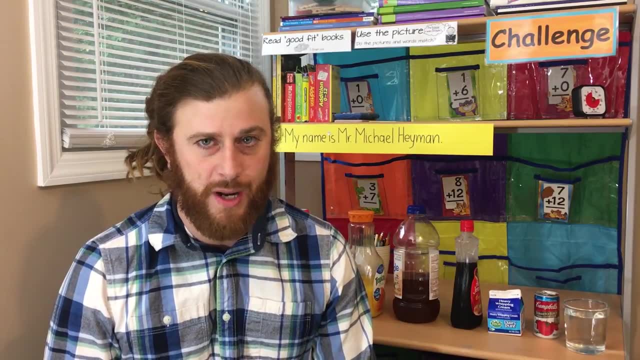 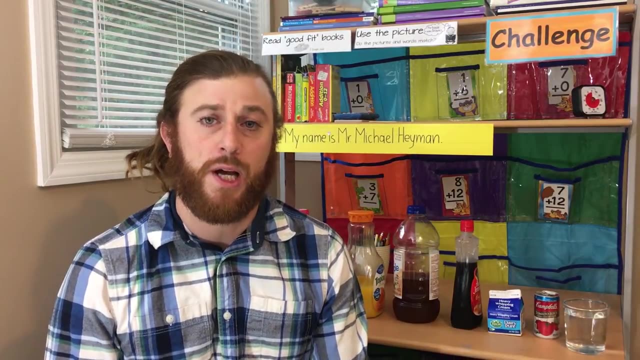 We've used an ice cube tray to make sure of this. Keeping track of your controls are a very important part of conducting a good experiment. Another part of conducting an experiment- maybe the most fun part- are the variables. In our experiment, the variables are the different liquids that we will freeze. 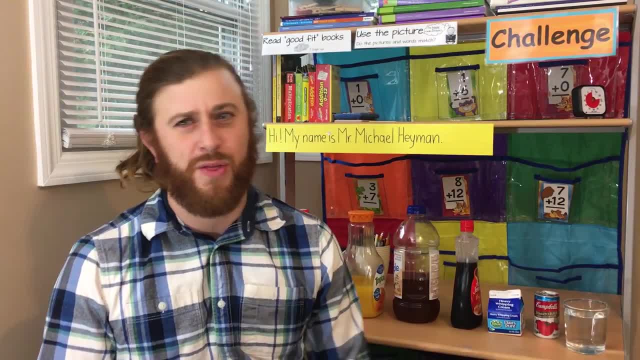 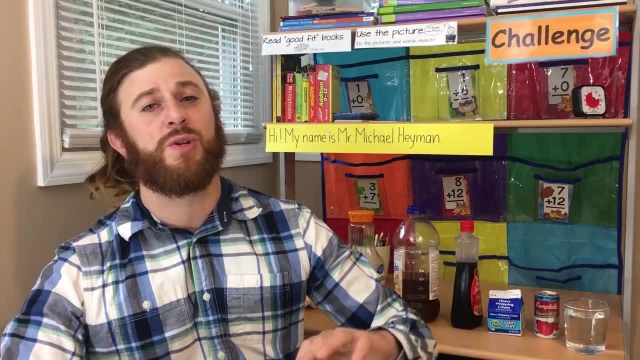 Now, as I've discussed before, for kindergartners and third graders and all students in between, you'll want to choose your liquids carefully First. you might want to say we're going to choose some liquids as a class and choose some nice easy liquids. 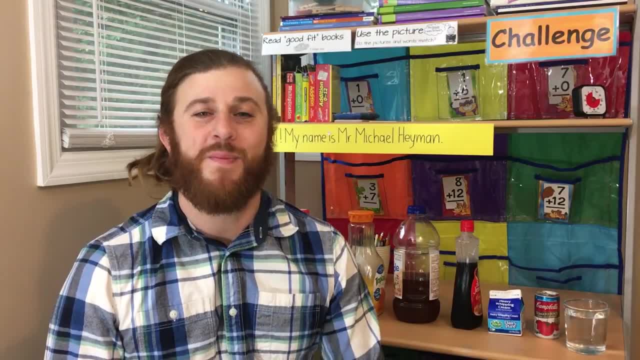 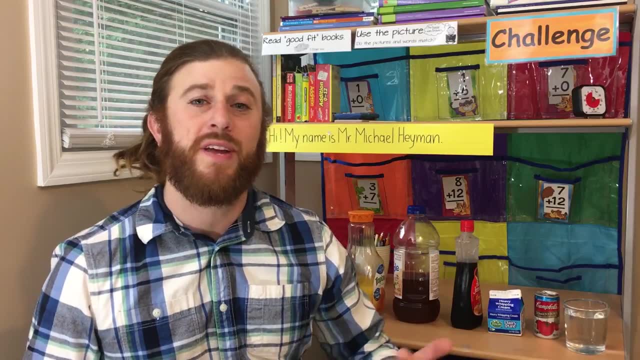 as we said, milk, orange juice and water. But then, to make it fun, students can choose their own liquids, and then they can ask even more complex questions, Such as: will this liquid even freeze in the first place? Choosing liquids such as maple syrup. 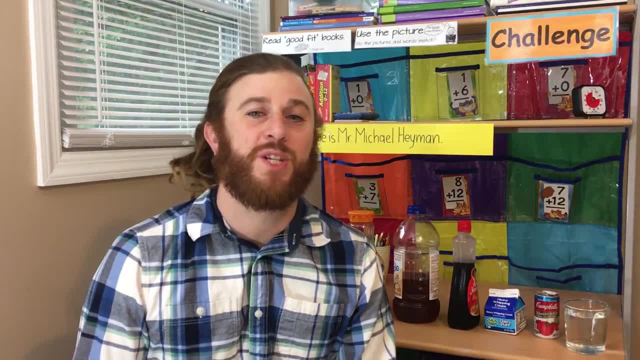 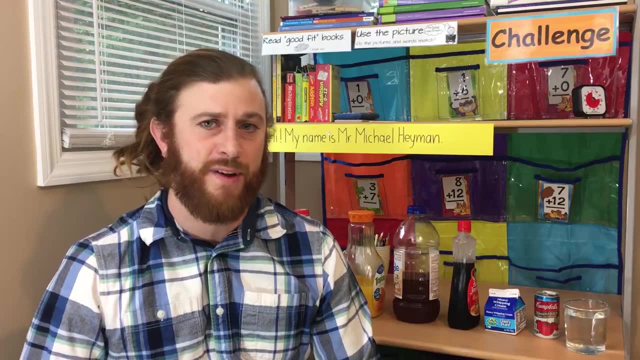 heavy whipping cream and tomato juice can help make these experiments a lot more interesting, especially if the students are the ones choosing the liquids. They'll always have more ownership of an activity if they're the ones making the decisions. We just took our ice cubes out of the freezer. 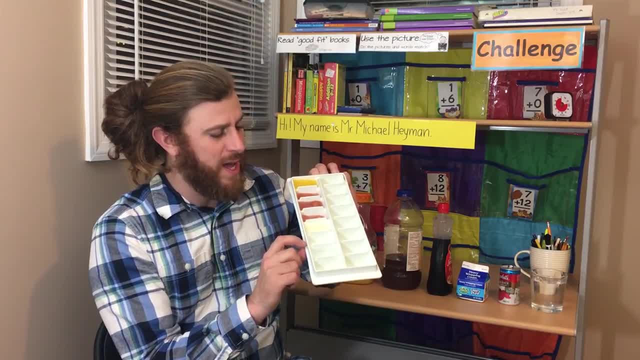 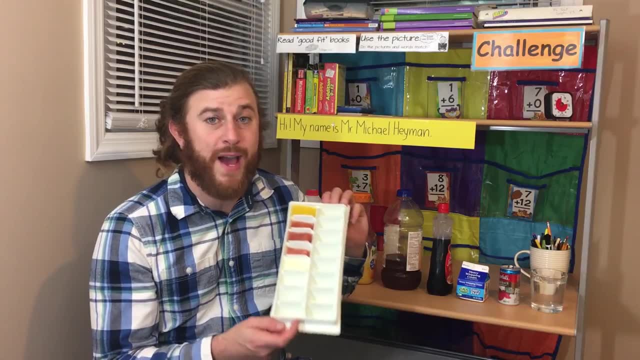 We have orange juice, iced tea, milk and water. Which one do you think is going to melt the fastest? As soon as we put these ice cubes in the bowl, we'll start the timer right away. We've controlled things like the temperature in the room. 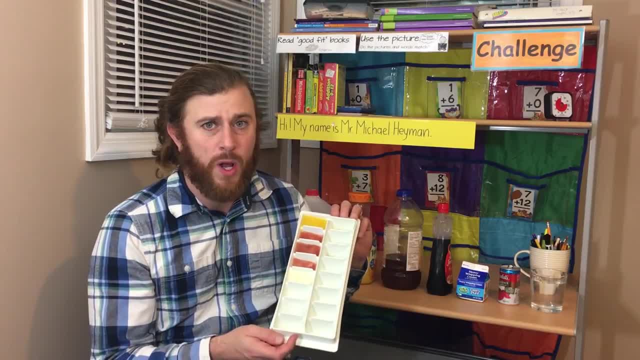 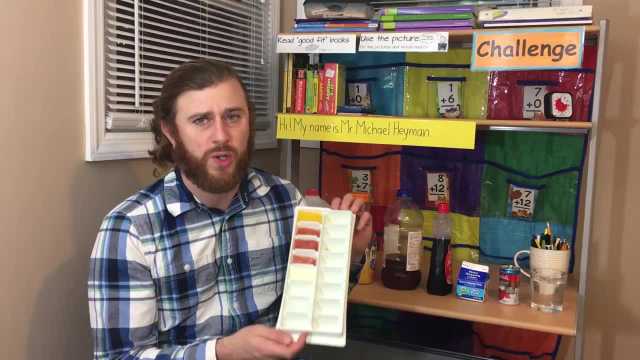 and the time. we've taken all the ice cubes out of the freezer. Now it's our turn to observe and see which ice cubes will melt the fastest. After they've all melted, we'll draw some conclusions and we'll report back with which ice cubes have melted the fastest. 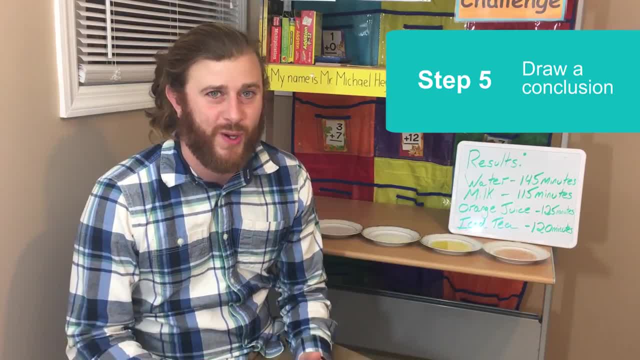 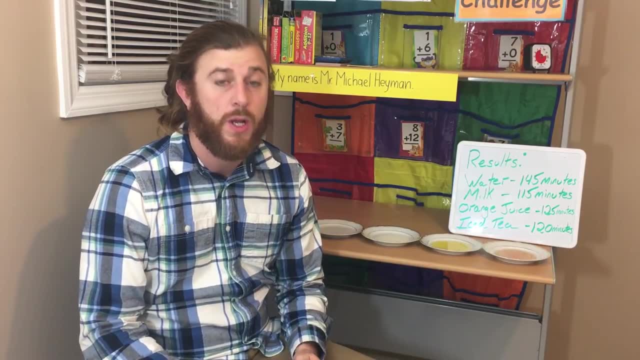 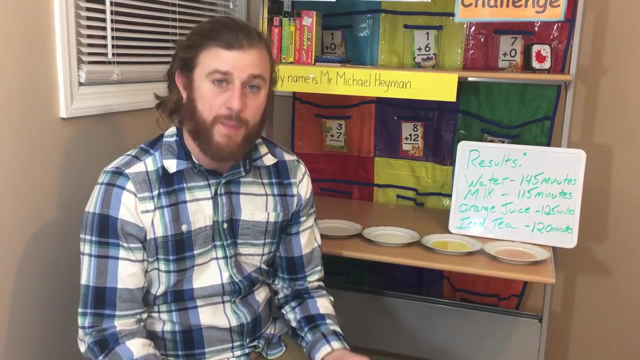 So we just finished our experiment and we have the results. We found out that milk melts faster than water, and orange juice and iced tea. This is our conclusion. We've found out our conclusion by conducting an experiment. This is the end of the scientific method.